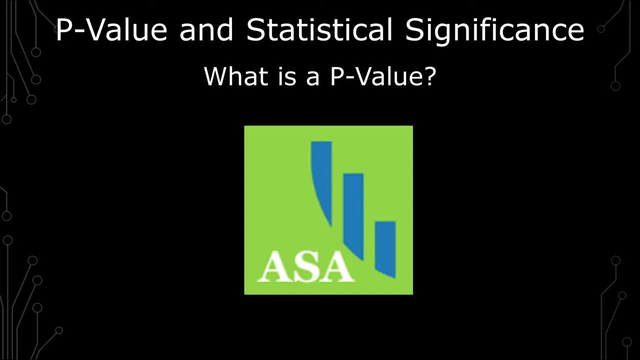 manner, And it wasn't just the you know Americans. It was actually a range of people from across the world that came down and sat and said: this is what a p-value is. The first principle is: p-values can indicate how incompatible the data are with a specified 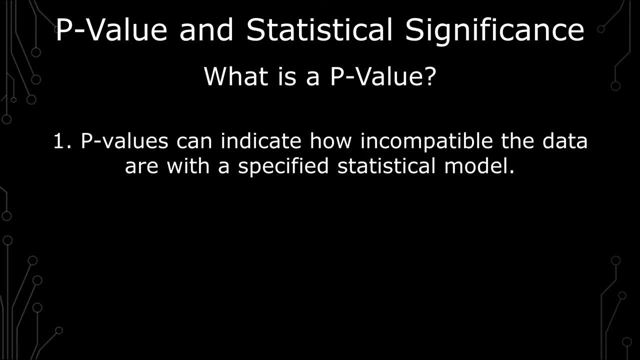 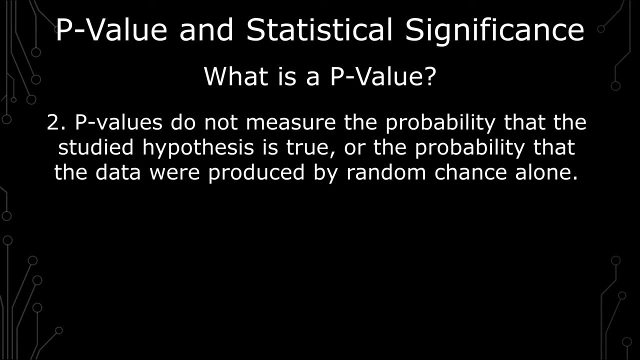 statistical model. So you're basically seeing, in regards to the null hypothesis, how compatible is the data that you've observed with that null hypothesis. The second is: p-values do not measure the probability that the studied hypothesis is true or that the probability that the data were produced by random chance alone. So this is to combat how a lot of people 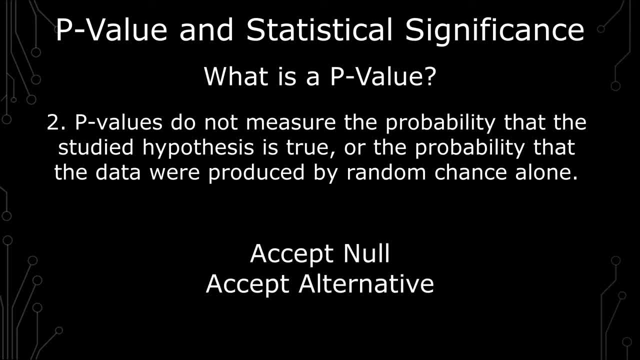 are saying accepting the null hypothesis, because by saying accepting the null hypothesis, you're actually saying a philosophical statement that it's true And a hypothesis can't actually state that. That's why, when you interpret hypotheses, it's fail to reject or reject the null hypothesis. 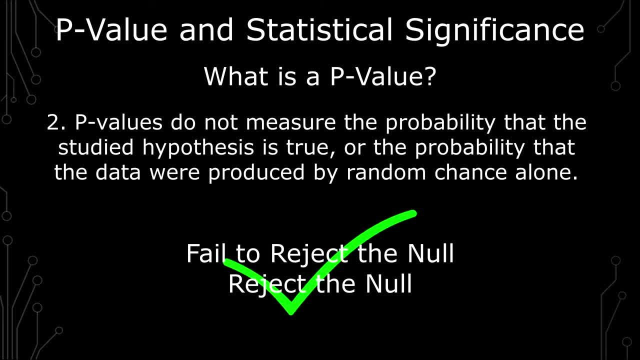 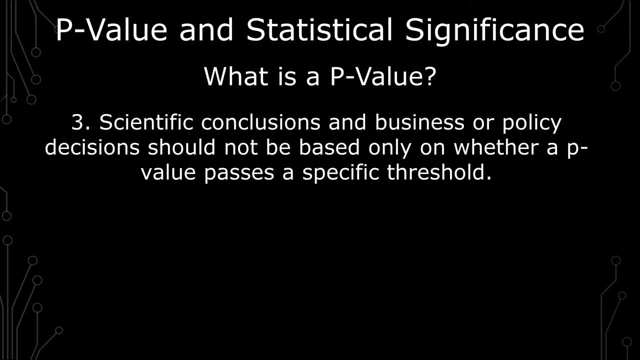 And you'll hear a lot of the time that the p-value is simply the probability of the data produced by random chance alone. That is also incorrect. The third principle is scientific conclusions and business or policy decisions should not be based only on whether a p-value passes a specified threshold. 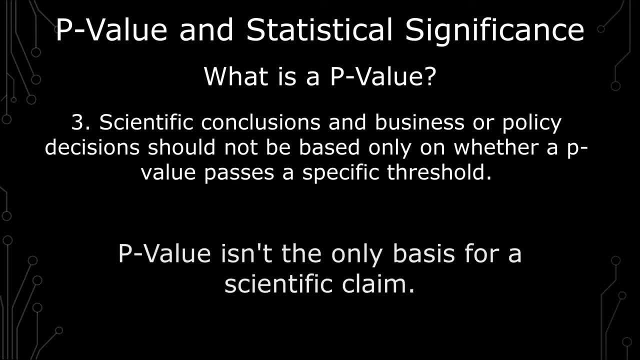 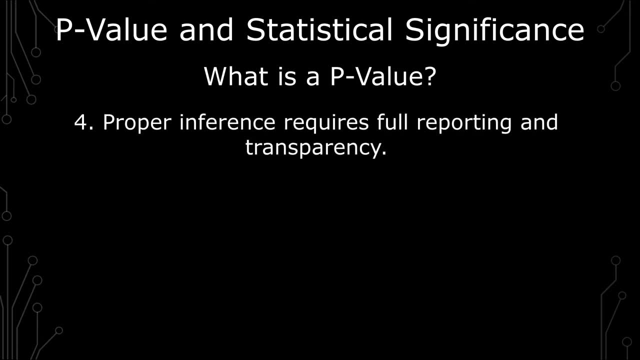 Another way of saying this is: the p-value shouldn't be the only basis for a scientific claim. You need to look at other things, such as the context or qualitative reasoning, the validity of statistical assumptions and the quality of observations and measurements. The fourth principle states: proper inference requires. 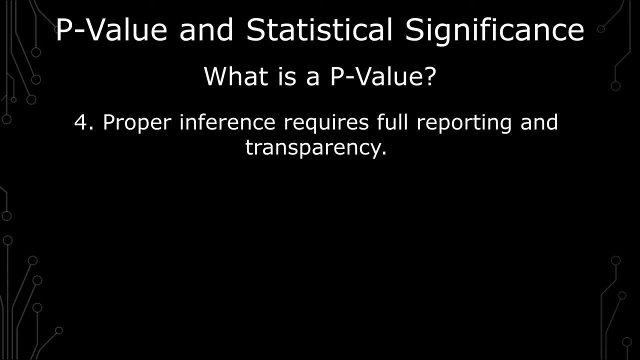 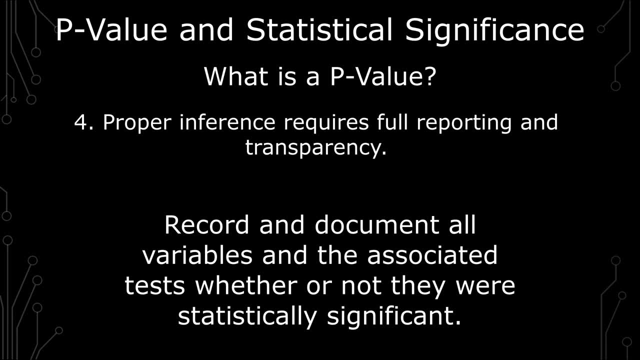 full reporting and transparency, And this has to do with the research articles themselves. So this is kind of a critique of the fact that if you have significant data, it would typically be published. If you didn't have significant data, it wouldn't be published. 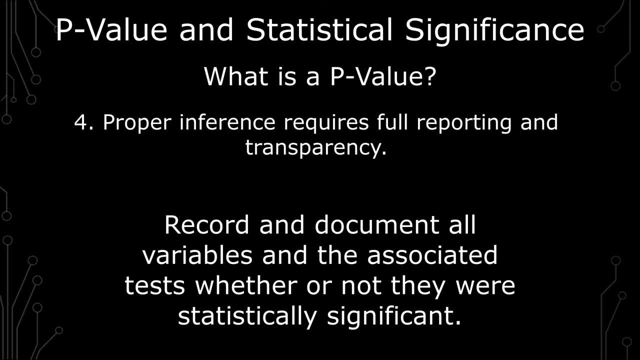 And that's inappropriate for a lot of reasons. One: maybe you have an idea and someone's already done it. You don't know they've done it because they weren't allowed to have their, their study published because the publishing firm or the journal wanted it to be significant statistically. 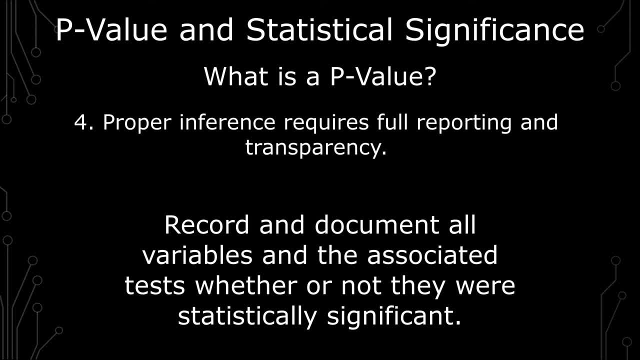 And that's just not appropriate in terms of scientific endeavors, because you end up with a lot of people wasting their time doing the same study over and, over and over again. So it's important to notate the variables that were not significant and to document what was significant and what wasn't. Number five is a p-value or statistical significance. 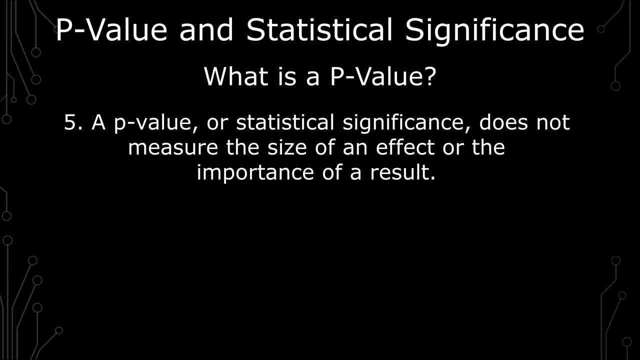 does not measure the size and effect or the importance of a result. That may be contrary to a lot of people's thinking. So the effect is obviously in most cases, especially if you're doing a regression, you're going to understand that the coefficient is what really measures the 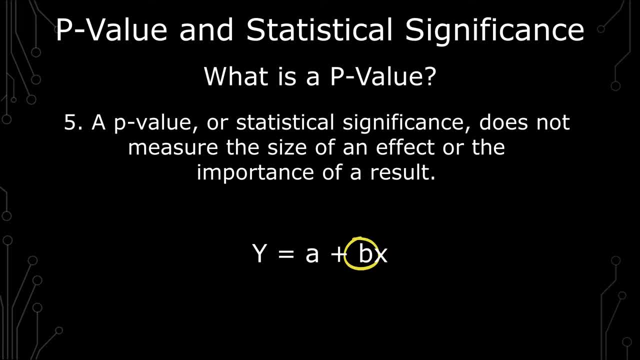 effect. The importance, though, that's different, And the reason why that's different is because the p-value is influenced by many factors, And sometimes it's simply a matter of sample size, Like, if you have a million observations, you'd probably have statistical significance in variables that had you only had a thousand. 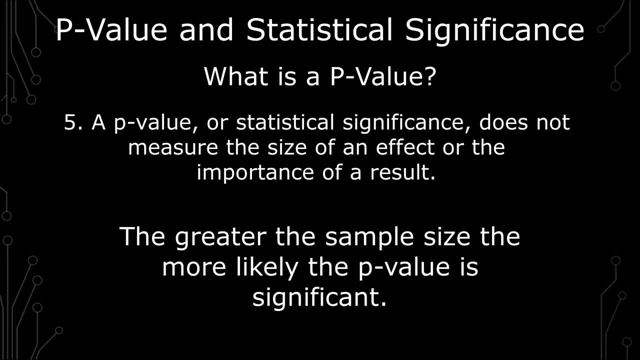 you wouldn't be able to have statistical significance. So it's important to understand what influences a p-value, and definitely sample size is one of them. You need to take several things into account when looking at a p-value And, in the context of those things, the p-value. 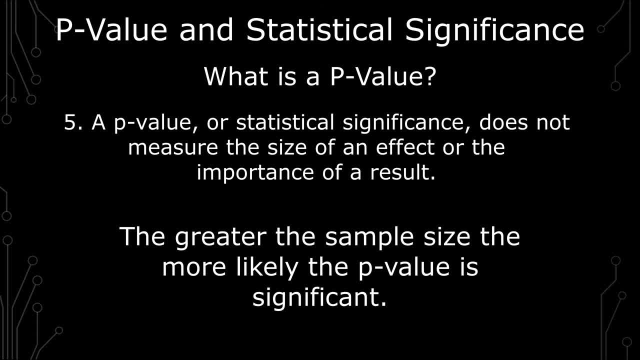 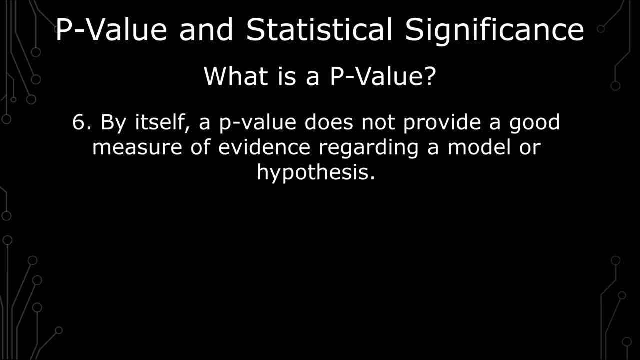 can be important, But without the context of those, a p-value by itself is not important, And that's what this is saying. So the last one: by itself, a p-value does not provide a good measure of evidence regarding a model or hypothesis. You really shouldn't just be checking a model. 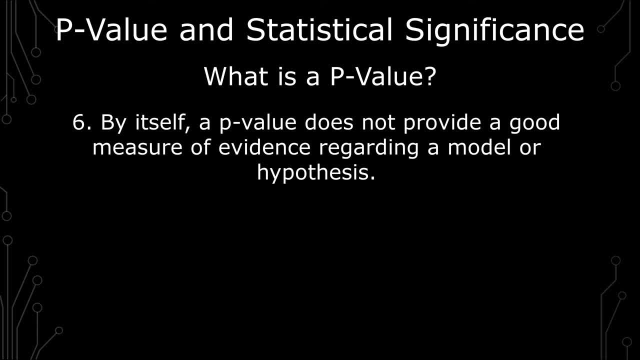 with a p-value. You should be checking a model with a p-value and the confidence or credibility or prediction intervals. You may want to use Bayesian methods. It depends on what you're looking at. So basically, it's about validating that p-value. That p-value cannot simply be by. 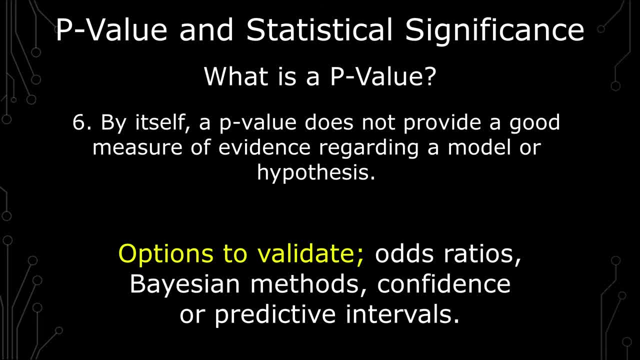 itself If you're using that p-value by itself, just like in principle five. it's not so much context here, though It's validation, And that you don't want to simply go off one piece of evidence. You want several pieces of evidence basically pointing in the same direction.